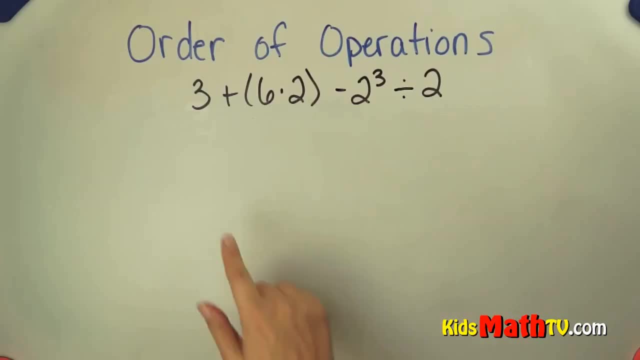 In this lesson we are going to use the order of operations to solve this expression. The order of operations To remember the order of operations I remember. please excuse my dear Aunt Sally, I know these are parentheses. E is for exponents. I multiply and divide. 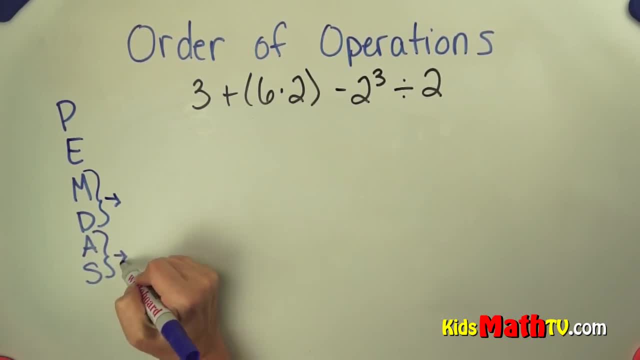 from left to right and then I add and subtract from left to right. You can write this on your paper and just remember. please excuse my dear Aunt Sally. I'm going to go in order of operations. First I'm going to look for parentheses and I see I have parentheses. 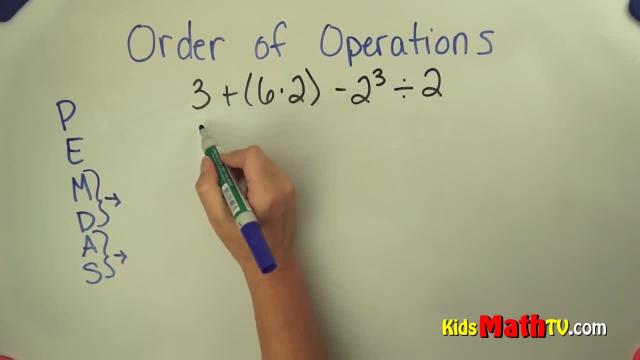 My next step, in my expression, is going to be 3+. I'm not doing anything with that, but I'm going to do this. 6 times 2 is 12.. I've evaluated the parentheses and I'm going to leave everything else the same. 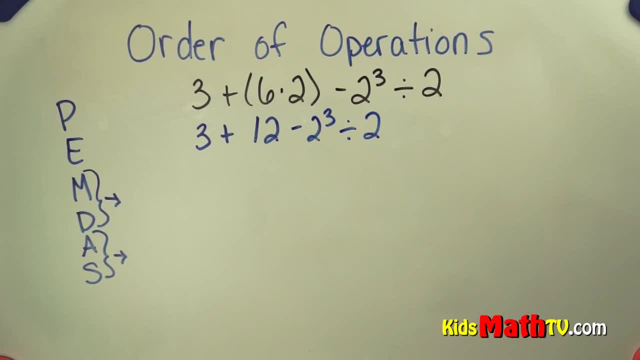 Okay, So that is my parentheses. Now I look I have no more parentheses. Do I have exponents? I do 2 to the 3rd, So I'm going to evaluate 2 to the 3rd. 2 to the 3rd is 2 times 2 times. 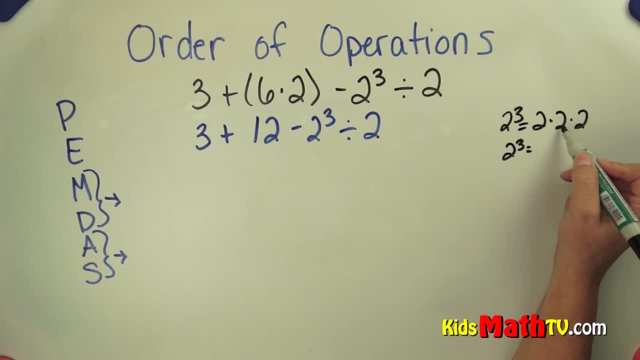 2, and 2 to the 3rd is 2 times 2 is 4, 4 times 2 is 8.. So I'm going to evaluate: Instead of 2 to the 3rd, I have 8.. So I'm going to leave: 3 plus 12 minus 2 to the 3rd is 8 divided. 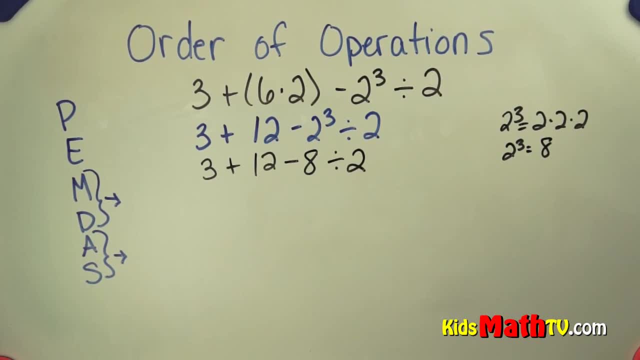 by 8.. Now I look to see if there's any multiplication or division, and I do that from left to right. I see that there is division. This division is right here: 8 divided by 2.. So I'm going to leave everything else- 3 plus, 12 minus- and just do: 8 divided by 2 is 4.. Okay. 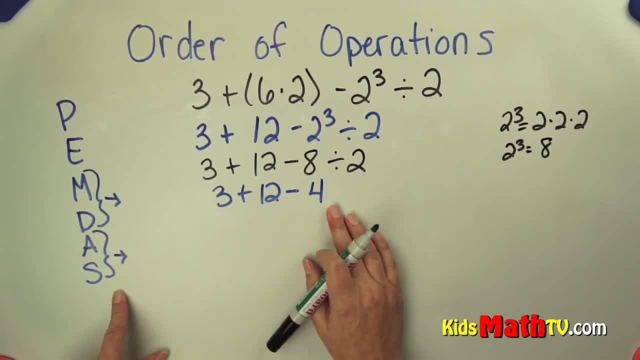 So I look: Is there any more multiplication or division? There is not. So now I add and subtract from left to right. I have to do the 3 plus 12 first. 3 plus 12 is 15 minus 4.. Now all I have left is subtraction. 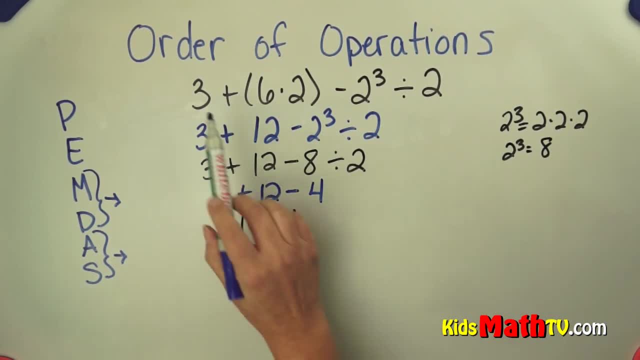 So 15 minus 4 is 11.. So the answer to this whole expression is 11. And it's the end of our lesson on order of operations.